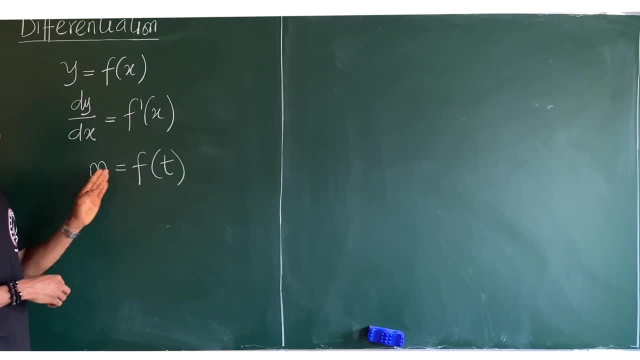 with respect to t is given by dm over dt, So it becomes dm over dt, which is changed in m with respect to t, or perhaps it's also equal in value to f prime of t. So this is just the very basic concept of differentiation: The change in a parameter with respect to another. 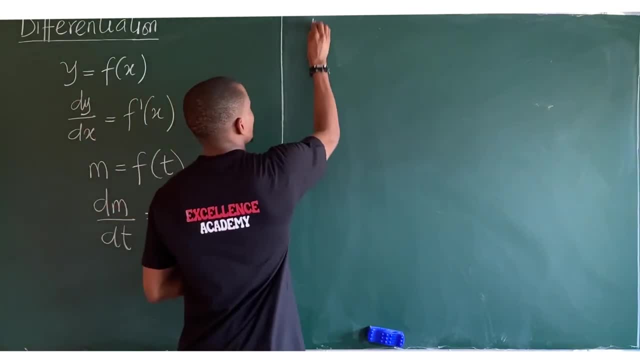 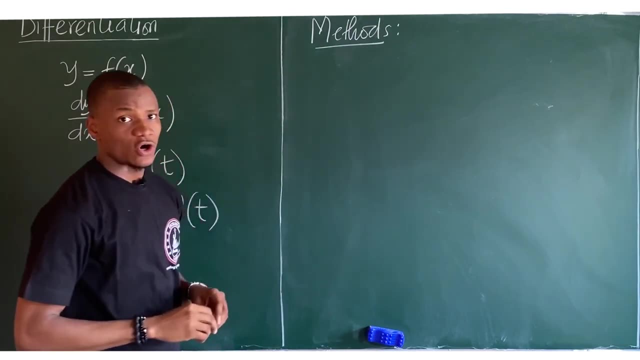 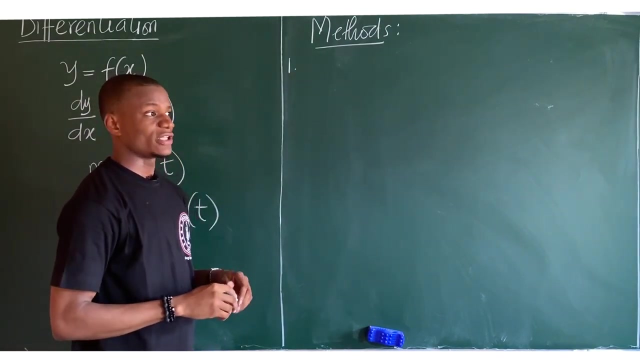 parameter. Having considered this, if I'm given a question to differentiate, what methods can I use? What are different methods of differentiation? There are about six methods of differentiation. We'll pick each of them and deal with them one after the other. The first method of differentiation: 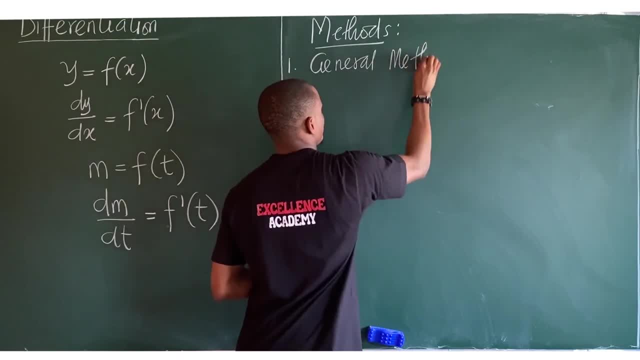 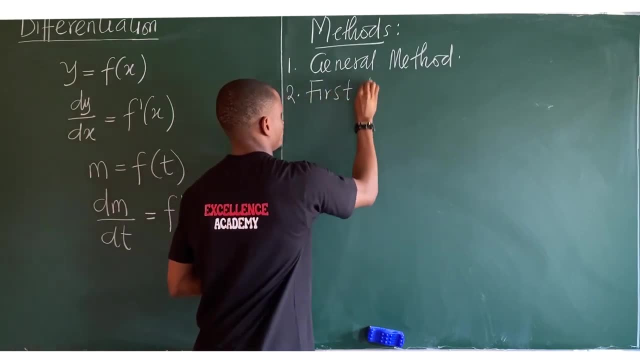 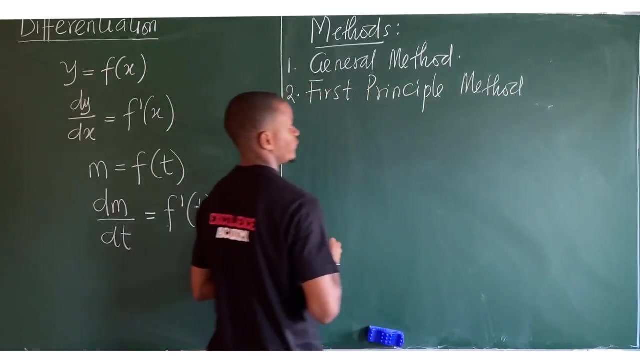 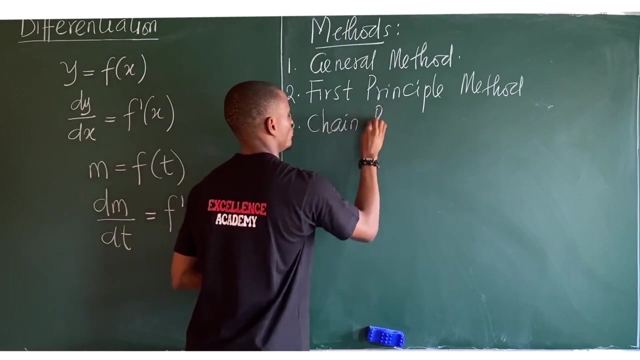 is known as the general method. Some prefer to call it the par method. Number two is known as the first principle method. That's my second method of differentiation. Number three is known as the chain rule. called the chain rule, Perhaps also referred to as the 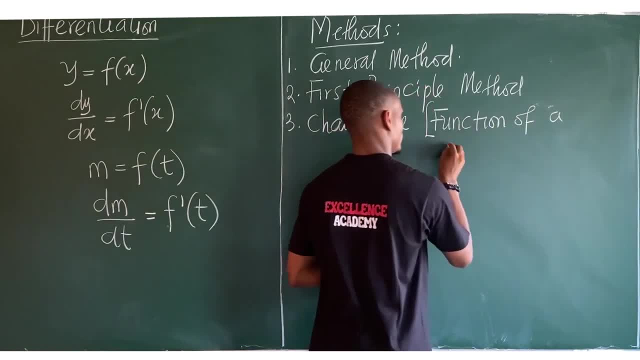 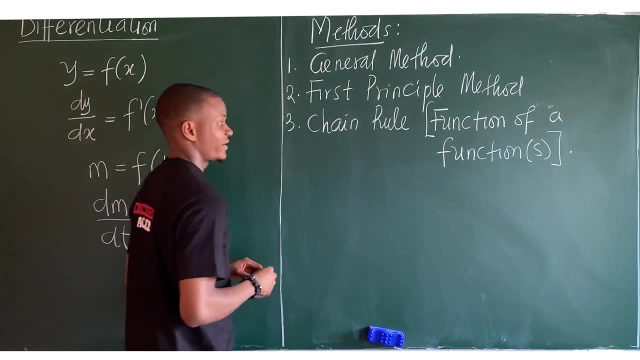 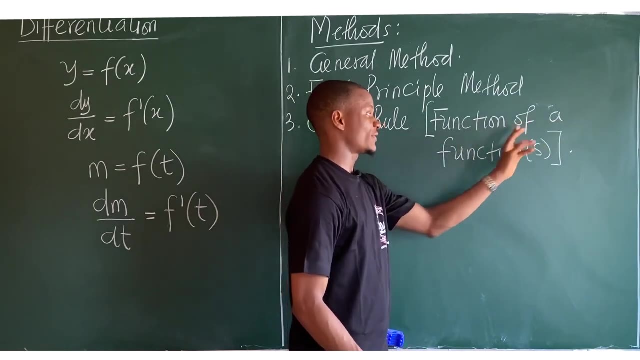 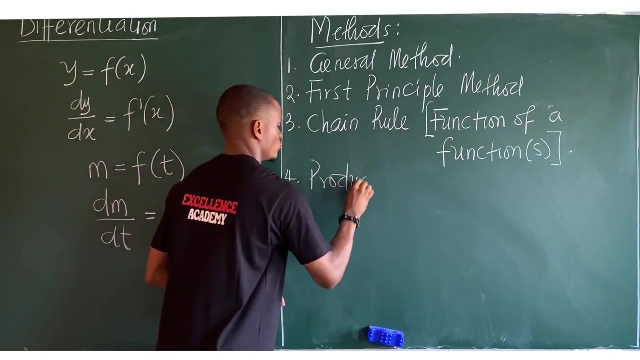 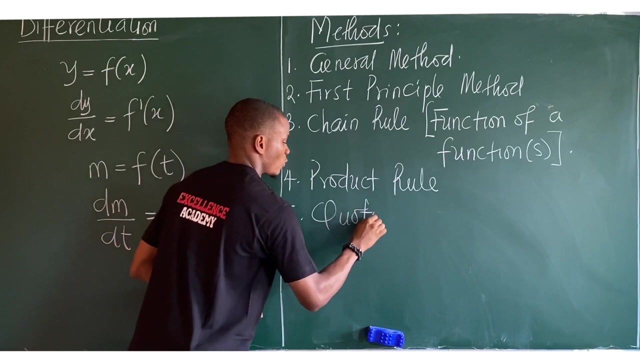 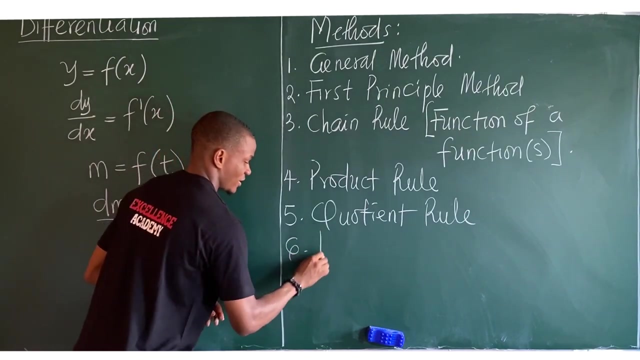 function of a function or function of several functions. So this is read: function of a function or functions of several functions. Number four: I have what is called the product rule. Number five: I have what is called the product rule, quotient rule, and one to this. number six: i have implicit differentiation. 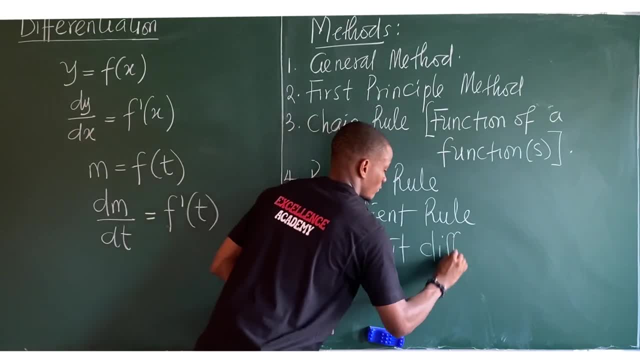 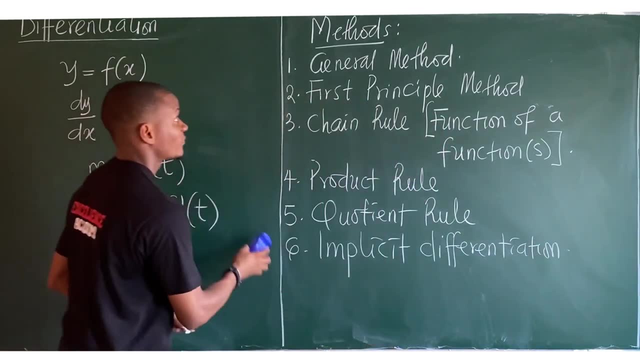 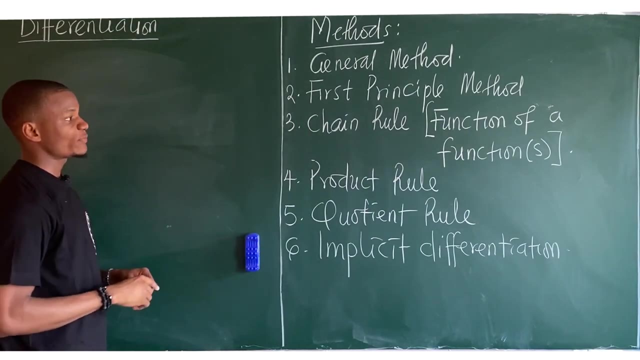 right. so these are like six different methods of differentiating terms. you have general method, you have first principle method. you have chain rule, also called function of a function or function of several functions- number four. you have the product rule- number five. you have the quotient rule- number six. you have implicit differentiation. let's pick up the first one. 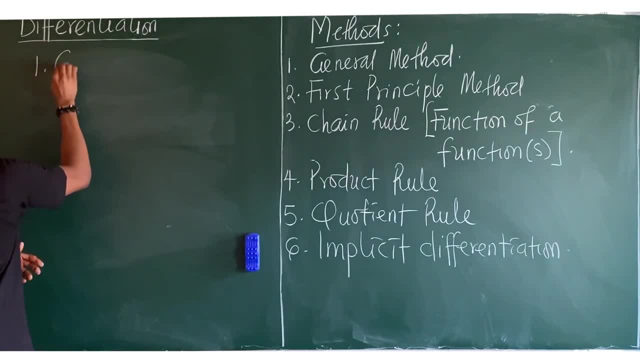 and explain this. the first one i have there is called the general method, general method of differentiation. how does this work? first up, let's assume i'm given a function y, i'm given a variable per se, y expressed as a function of x, f of x, and let's say: this is now equal to x to a particular power. 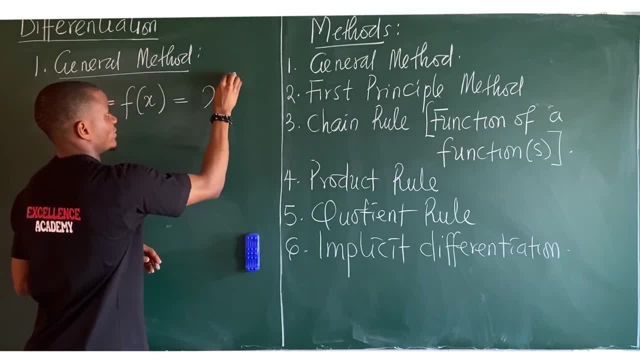 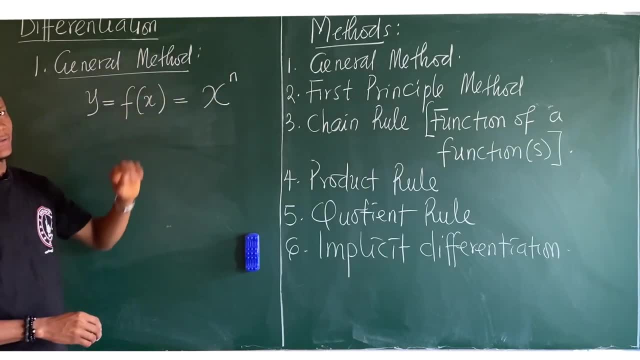 or a particular index, let's say n. all right, so i'm giving the function y being equal to f of x, such that this is equal to x power n. if i differentiate this now using general method, i will have that the y over the x is equal to. 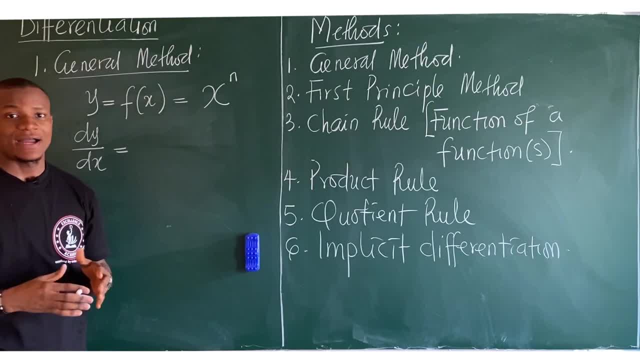 the idea is very simple: i will multiply by the power, i will subtract one from the power. so from this now i'm having x is called the base and n is called the power or the index or the degree. so multiply by the power. here that's n, so becomes n times. i'm having what i have here. 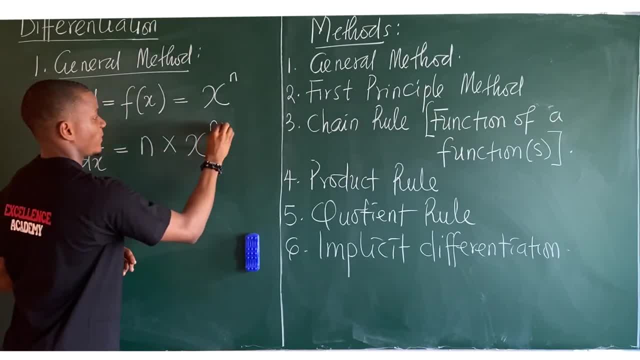 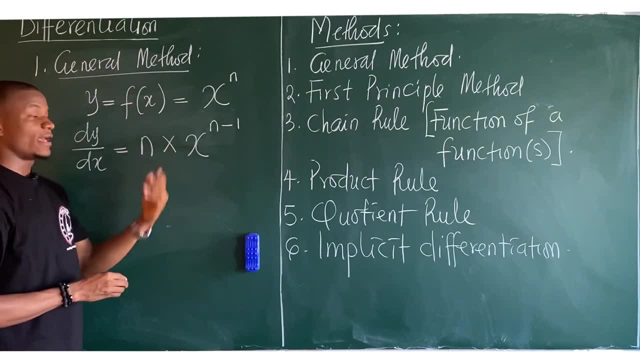 x by what? n subtracts 1 from the power. Please observe, I said multiply by the power, so n times this subtracts 1 from the power, n minus 1, such that if I work on this, it's now equal to n times x. 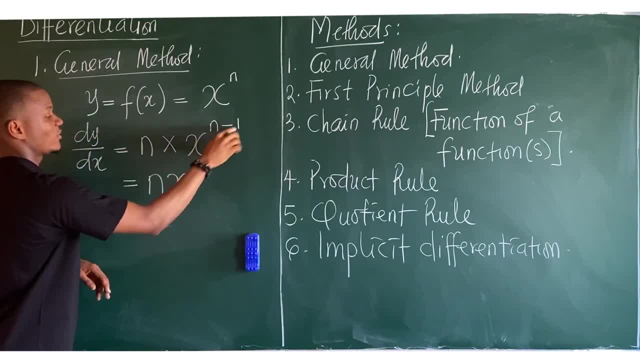 gives you nx to power, n minus 1,, of course, obviously n minus 1.. So here's the little concept of general method of differentiation. I'll pick an example and buttress this point. Let's say I have that y is equal to x to power 3, right, If I differentiate this, I'll have that. 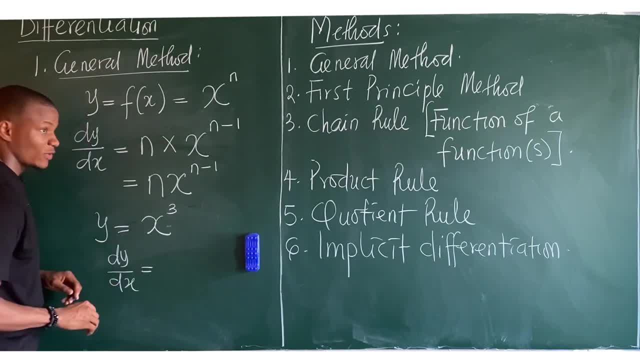 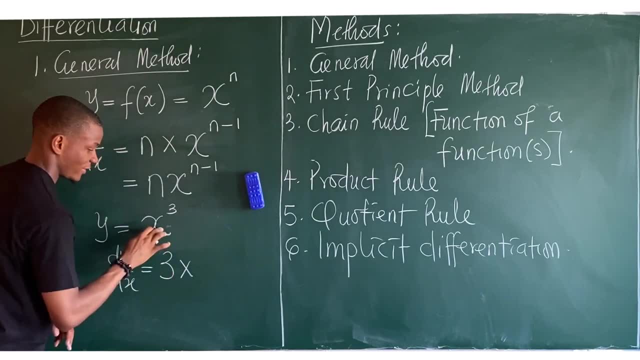 dy all over. dx is equal to the power. here is 3, so it becomes 3 times this. so I'm having 3 times what I have here, that's x to power 3, we said subtracts 1, becomes minus 1, this is now equal to: I'm having 3 times x is 3x. 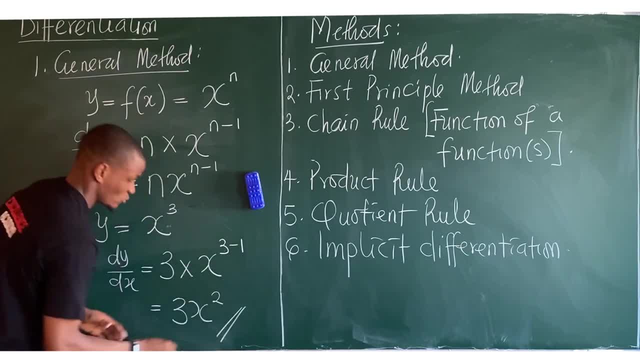 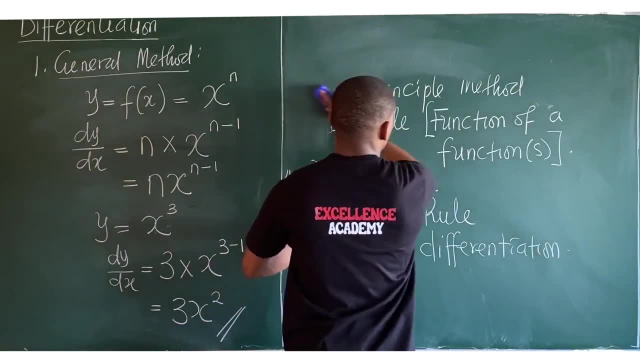 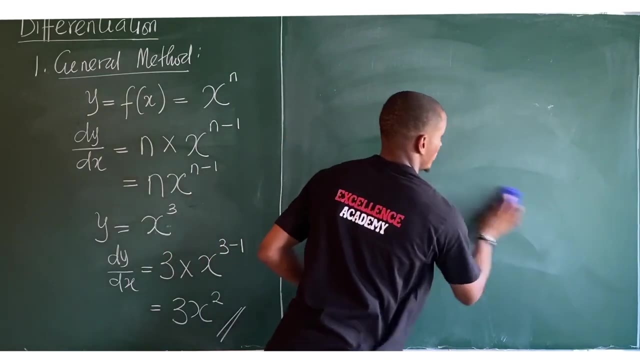 into 3 minus 1, that gives you 2.. So this is the simple answer for this right. So look at- we'll take other examples and look at much more cases. on general method, Don't forget the concept is very simple: multiply by the power and subtract 1 from the power. 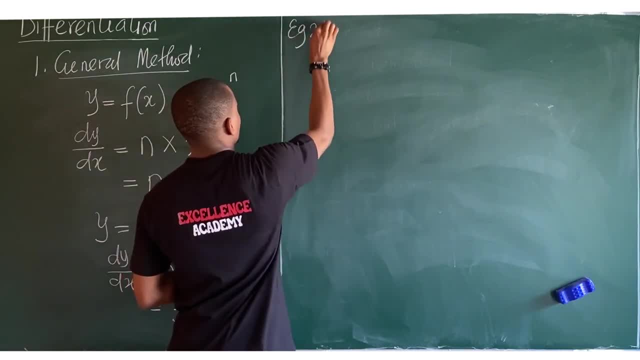 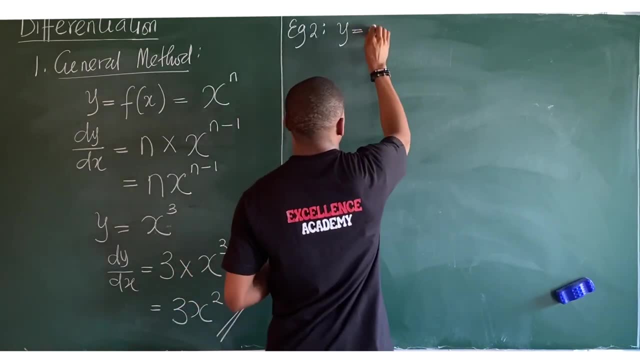 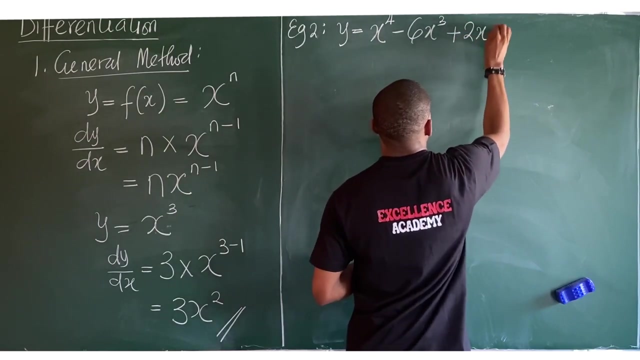 let's take a second example, example 2.. Let's assume I have a function, say y, being equal to, let's say x to power 4 minus 6x cubed plus 2x squared minus 8x plus 11.. 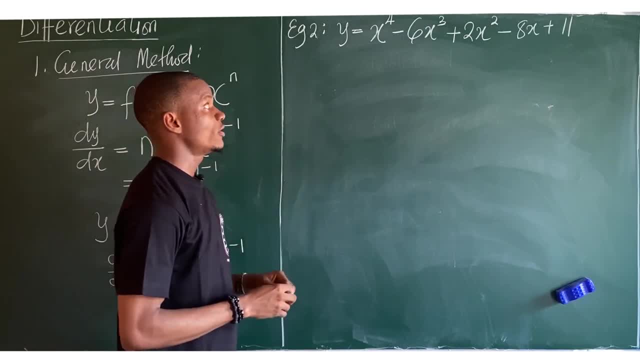 All right, let's say we have this, y being equal to x to power, 4 minus 6x, cubed plus 2x, squared minus 8x plus 1.. I'm asked to find dy over dx here. what do you do From this? 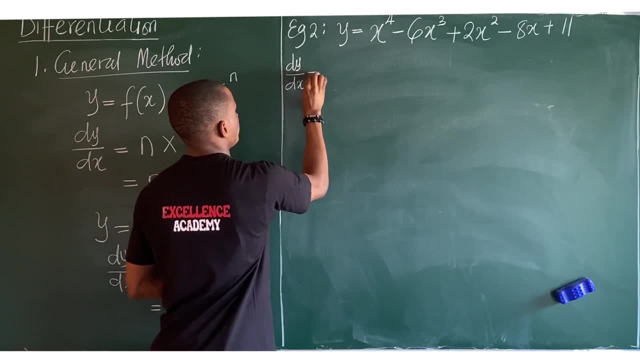 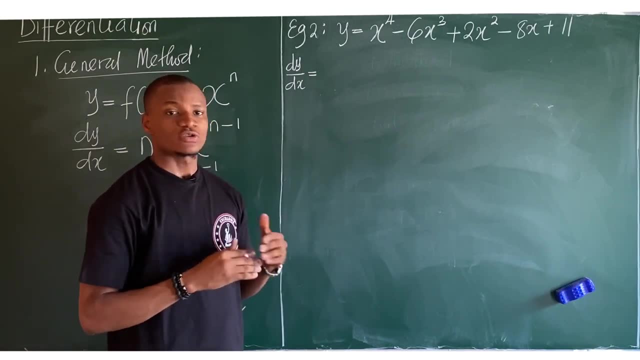 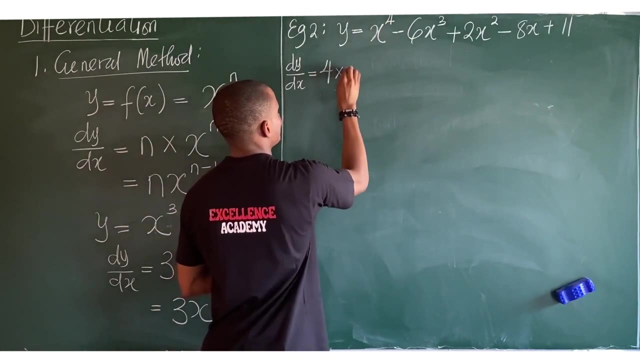 I'll have that dy all over. dx is equal to. I will use the same concept throughout all of this right. The concept is multiply by the power subtract 1 from the power From this here. the power here is 4, so becomes 4 times x into subtract 1, 4 minus 1.. Next up, I have a minus. 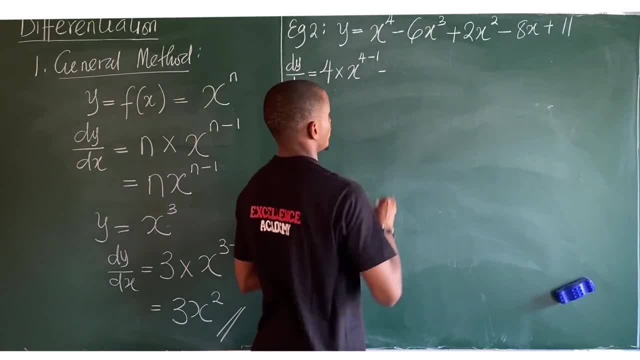 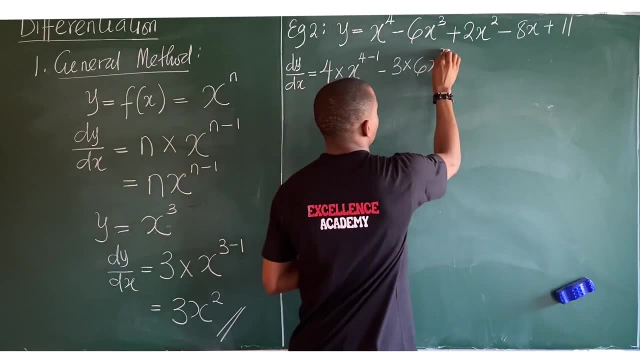 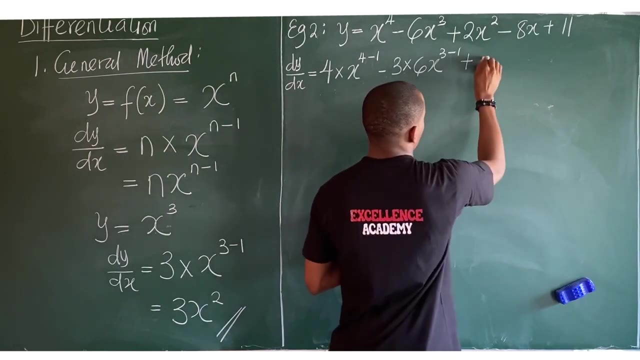 here. so it becomes minus. the power here is 3, so it becomes 3 times what I have here, 6x into this, 3 minus 1 plus next up, the power here is 2, so it becomes what there, 2 times. 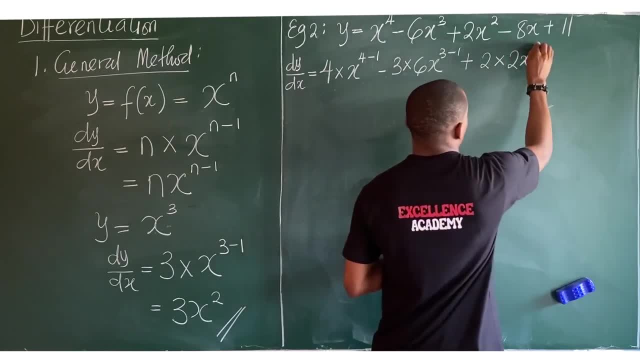 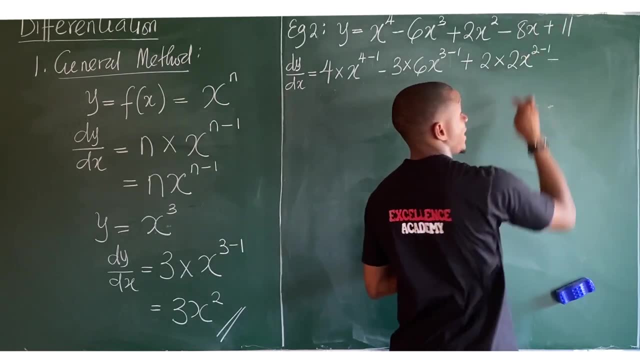 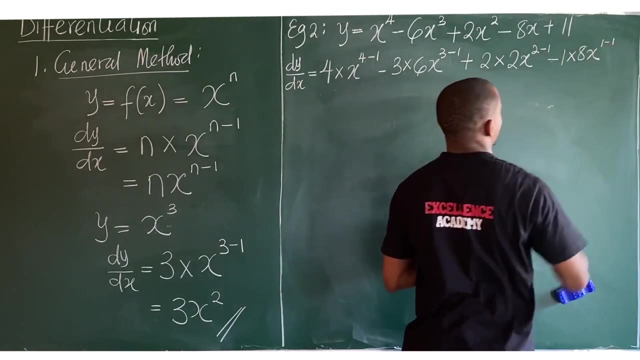 what do you have here? 2x into what I have here, 2 minus 1.. Next up minus, I'm having 8x here. the power here is 1, so it becomes 1 times 8x into what there: 1 minus 1.. Finally, 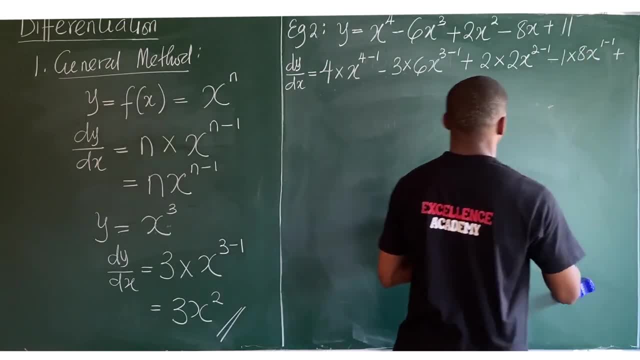 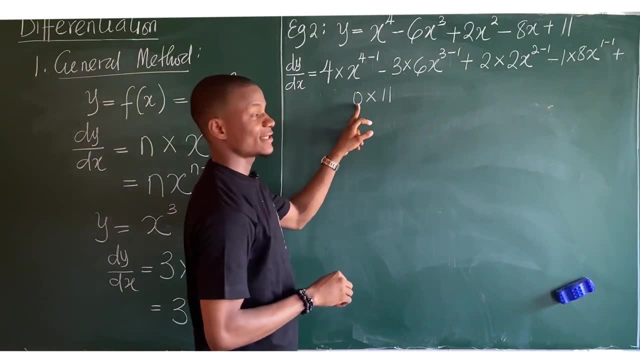 plus, I'm having a constant here. it becomes 0 times 11.. Now question: why is this a 0? Why do I have a 0 here? You could say: I'm having a 0 here because there is no x. 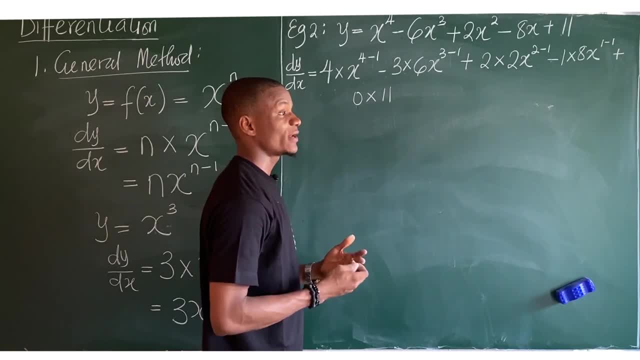 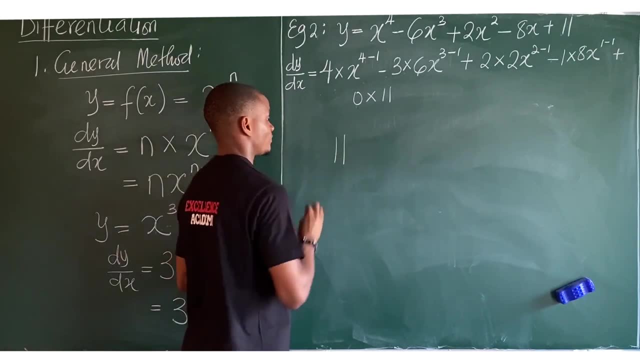 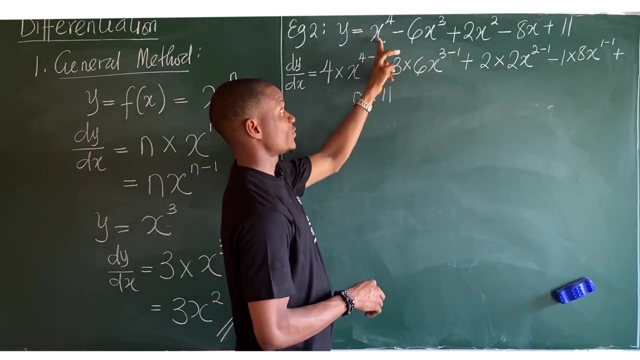 attached to it. it's called a constant. For a constant, multiply the value there by 0.. Why is this? so I'll explain this. Let's say I have 11 here. Now if you observe through this polynomial, you observe that I'm having x attached to each of the terms there. So this is x to power 4,. 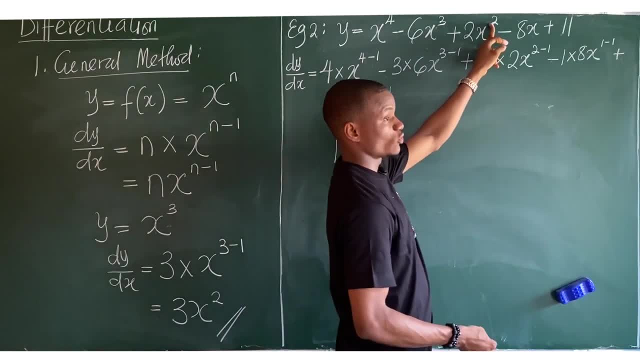 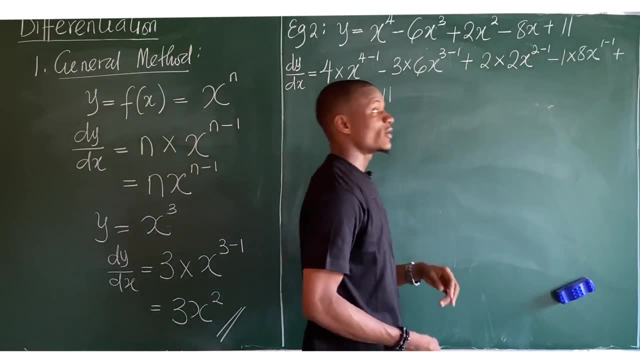 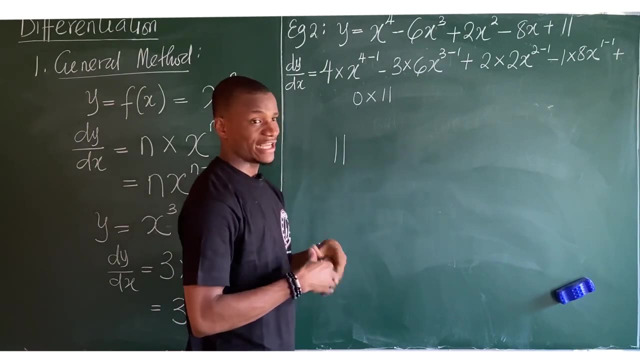 x to power 3, perhaps x cubed, x to power 2, x squared. I'm having x here, So x is attached to all of these terms here except 11.. Now, if I have 11 standing alone, is there an x attached to it? Yes, we could express 11 in terms of x. 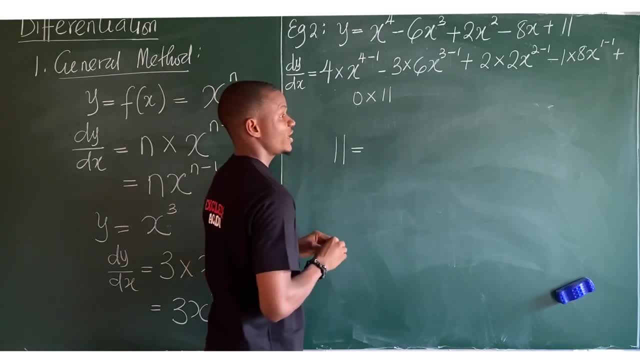 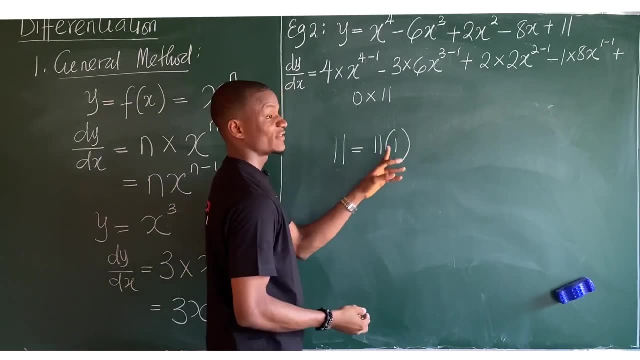 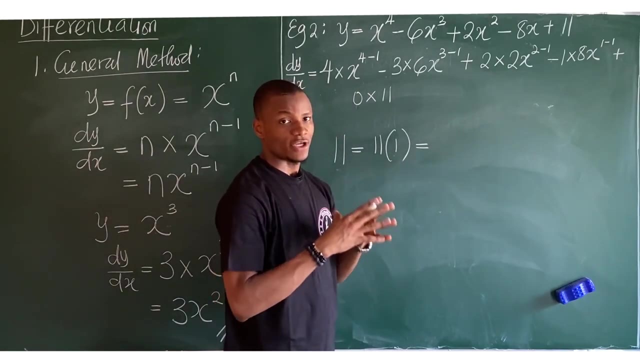 How, If I have 11, we could say: 11 is equal to what there 11 times 1.. So 11 is same as 11 times 1.. I can express 1 in terms of x Using the zeroth law of indices. From the zeroth law of indices. we have that, anything or any. 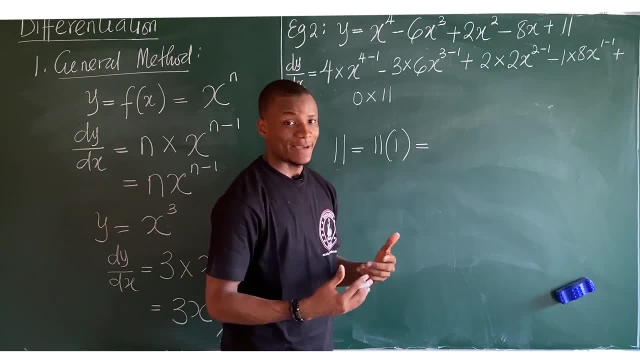 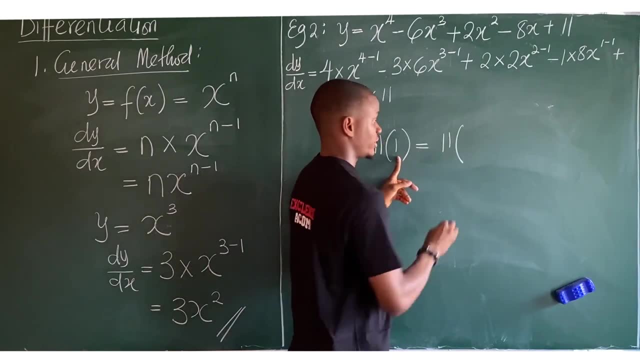 number raised to power 0 is 1 except 0.. All right, So it's now equal to 11, 1 in terms of x gives you what there? x to power, what 0. So x to power 0 is still 1.. So if I work on this, 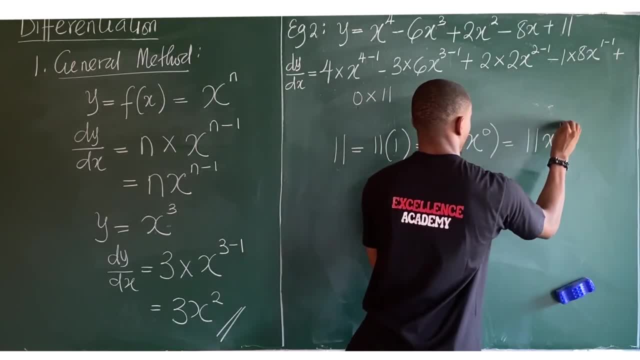 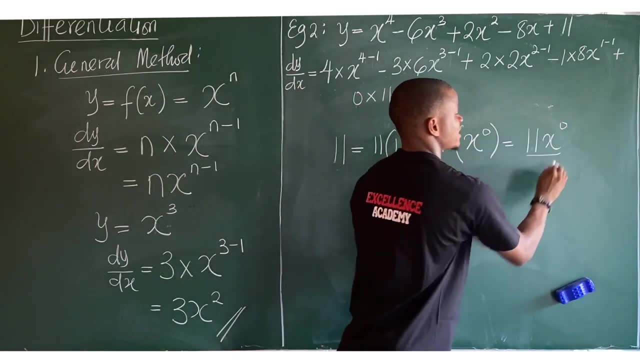 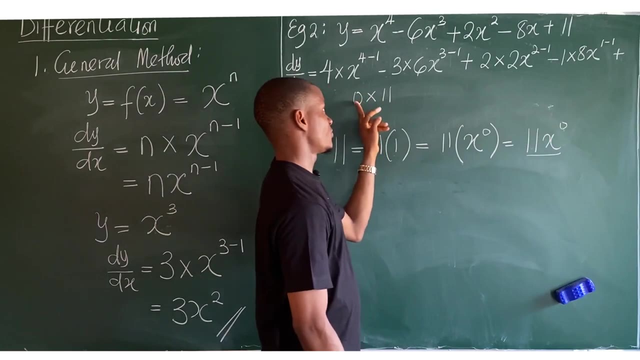 this is now equal to 11 x to power 0. Hence 11 is the same thing, That's 11 x to power 0. So if I employ this method, using general method, we said multiply by the power. The power here is 0. So it becomes 0 times 11.. So that's how I got 0 times 11.. 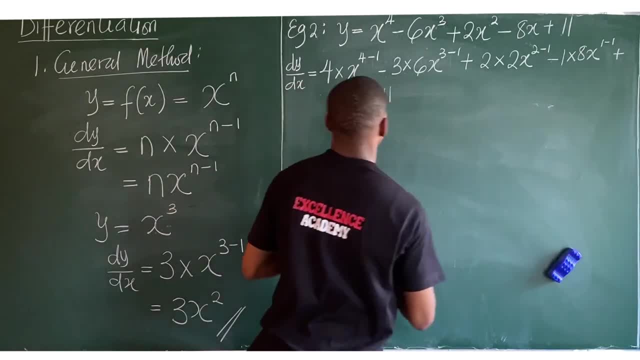 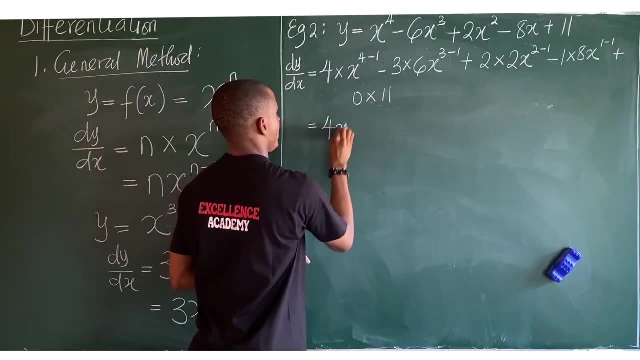 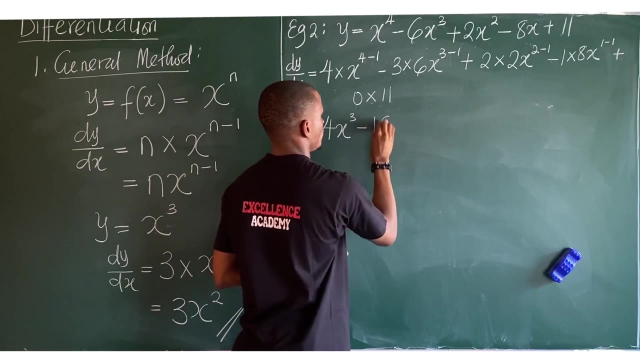 All right. So next up from this now, I'm now having equal to, I'm having 4 times x. That gives you 4 x into 4 minus 1.. That's 3.. Plus 3 times 6 gives you 18 x into 3 minus 1.. That's 2.. 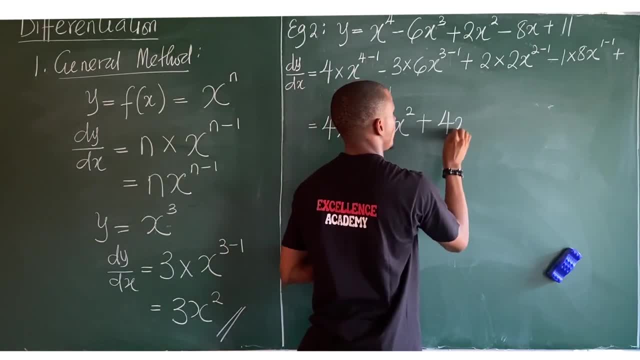 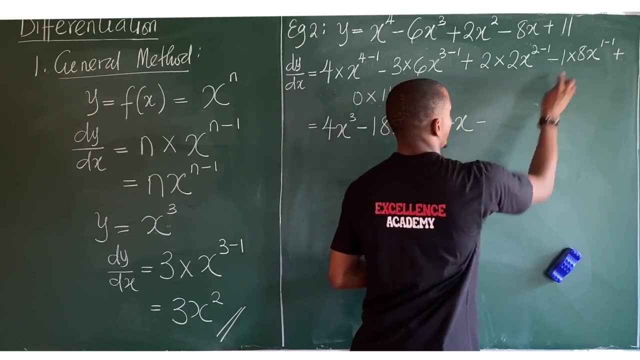 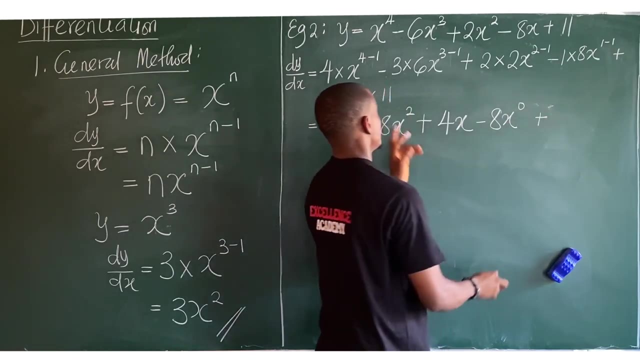 Plus, next up, 2 times 2 gives you 4 x into 2 minus 1 is 1.. That's 4 x Minus 1 times 8 is 8. x into 1 minus 1 is 0.. Finally, plus 0 times 11, obviously is 0.. 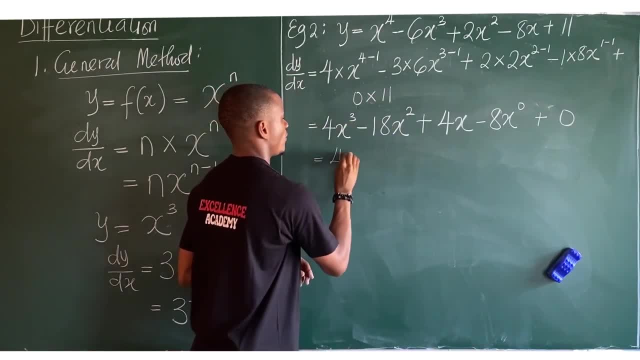 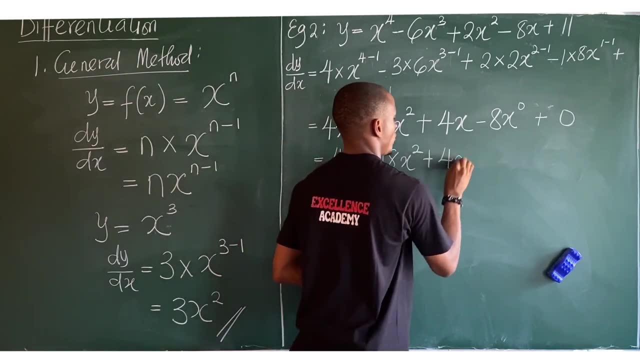 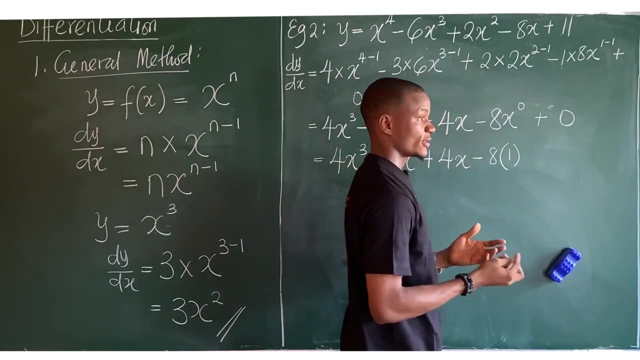 So if I work on this now, it's now equal to I'm having 4 x cubed minus 18 x squared, plus 4 x minus 8, into x to power 0. It gives you what there? 1 plus 0. It's off x to power. 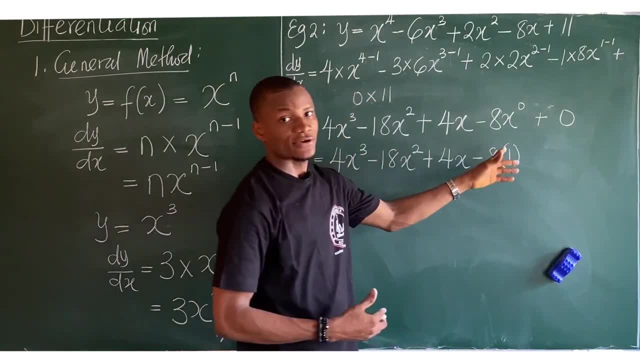 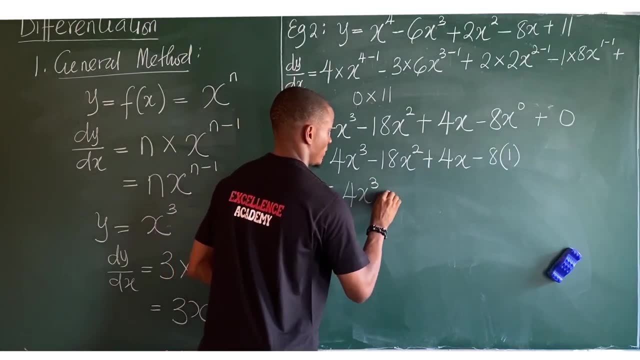 0 is 1.. From the z-th law of indices into x to power. 0 is what? 1.. All right, So this is now equal to 4 x cubed minus 1. That's 1.. So this is now equal to 4 x cubed minus. 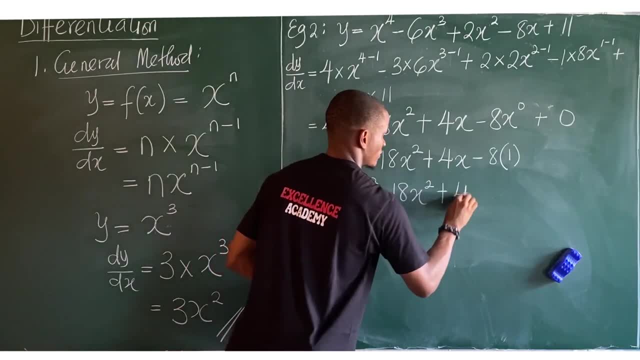 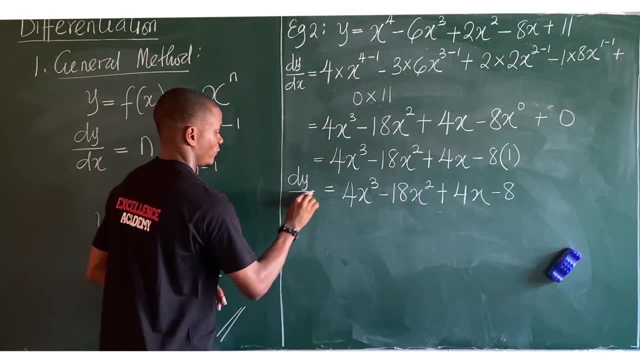 18 x squared plus 4 x minus 8 times 1. Gives you what there Minus 8.. So hence this becomes the value for dy over dx. Looking at this, I can see like terms. These are even: 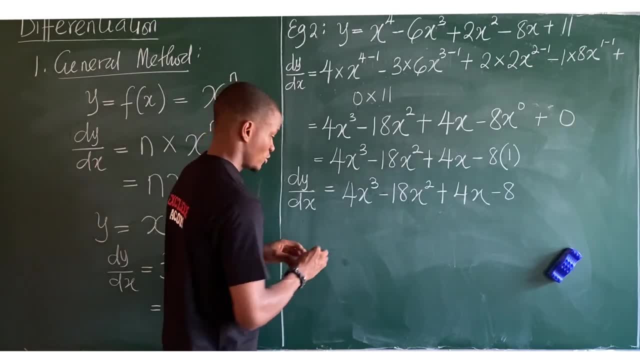 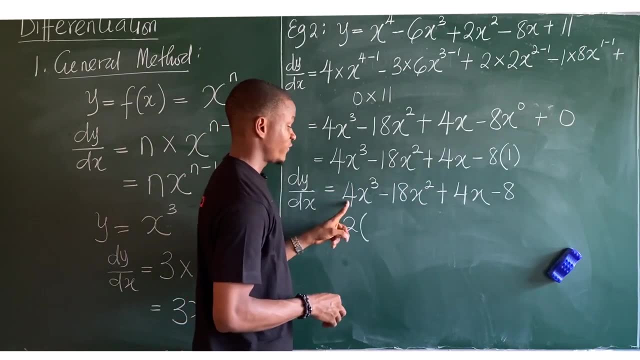 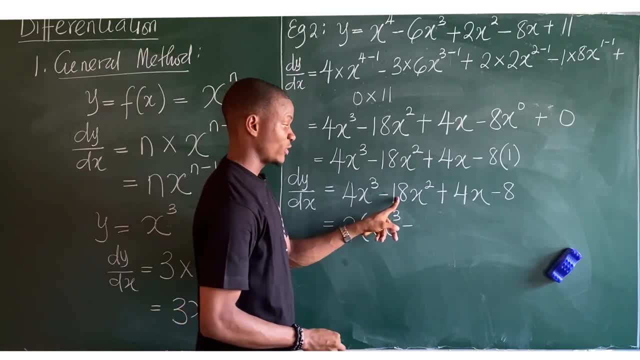 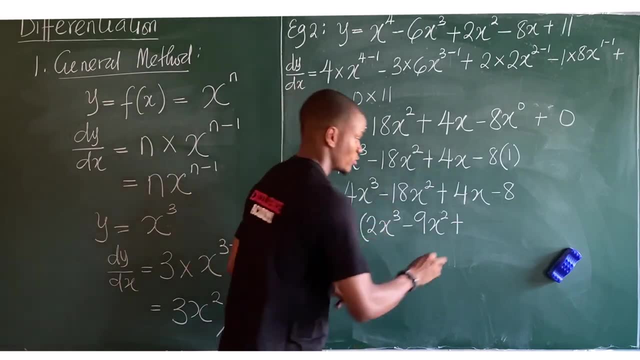 3. Minus. Here's 18 divided by 2. You have what there? Having 9 x squared plus, Here is 4 divided by 2. You have what there? 2. So it gives you 2 x minus. Here is 8 divided. 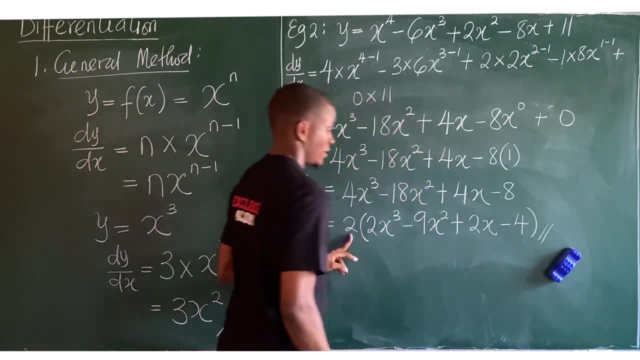 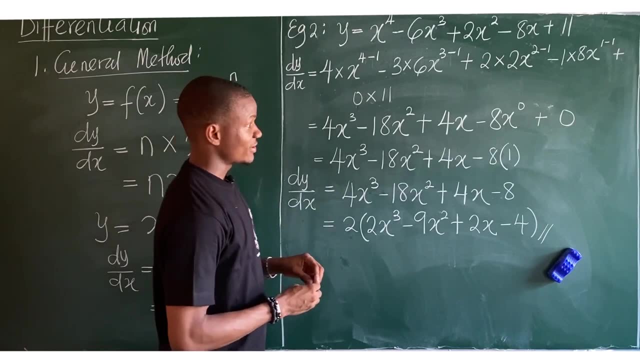 by 2.. You have what there? 4. So this becomes the factorized value for my dy over dx. Now for this. now I want you to observe two things. Number 1 is this: That if I differentiate a term such that it's just that term and x. 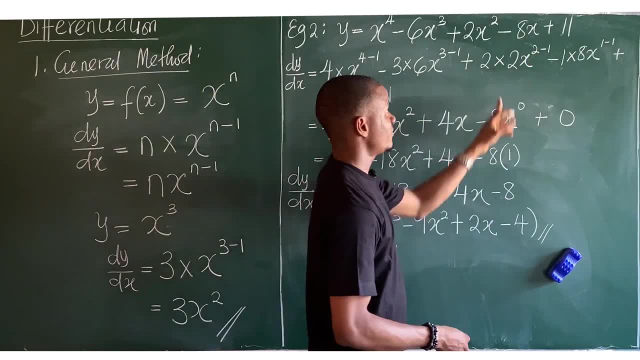 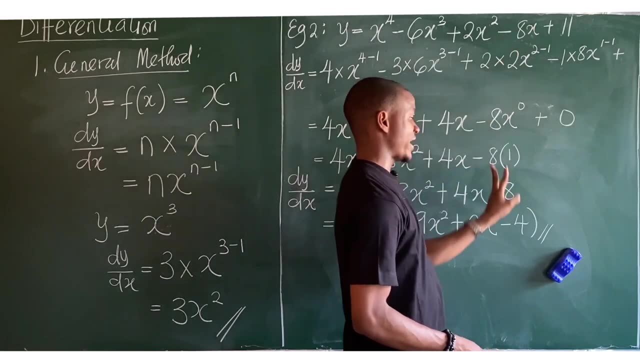 At the end it gives me that term. So I'm having minus 8 x here. If I differentiate minus 8 x, it becomes just this term and x to power 1. It gives you at the end minus 8.. Next up, if I differentiate a constant, that means a term without x. there it gives. 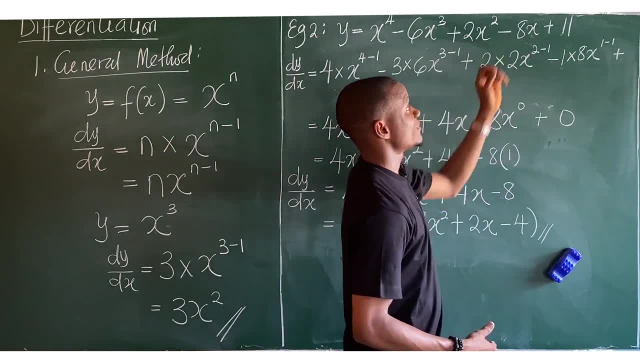 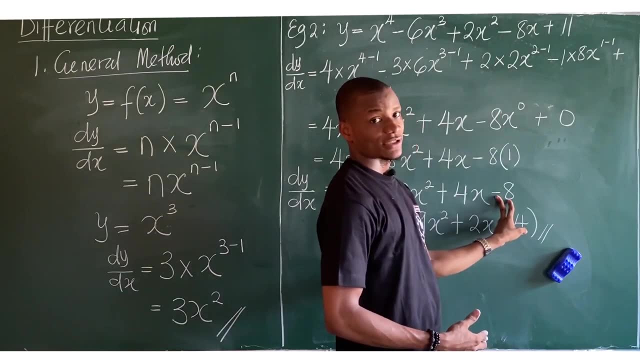 me 0.. So know these two things please. If I differentiate a term such that it's just that term and x to power 1, at the end of the differentiation process it gives you that same term minus 8.. If I differentiate a constant, 11..